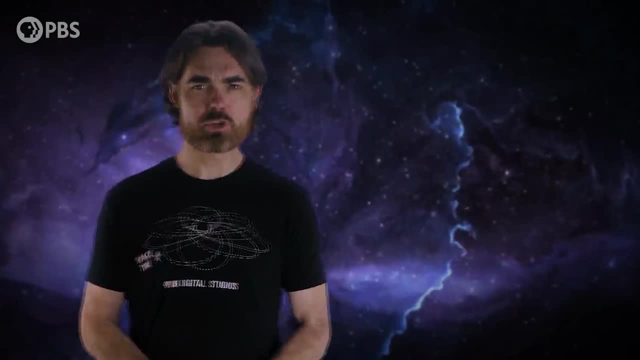 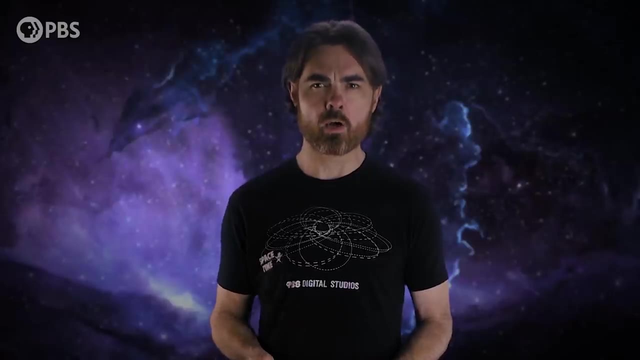 to solving the black hole information paradox, a solution that may one day unite quantum physics with gravity. But despite these clues of the importance of entropy in the second law, it is not obvious what makes it so fundamental. A system's entropy is what we call an emergent property. 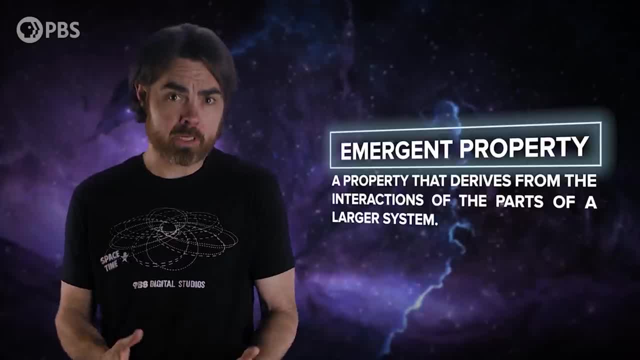 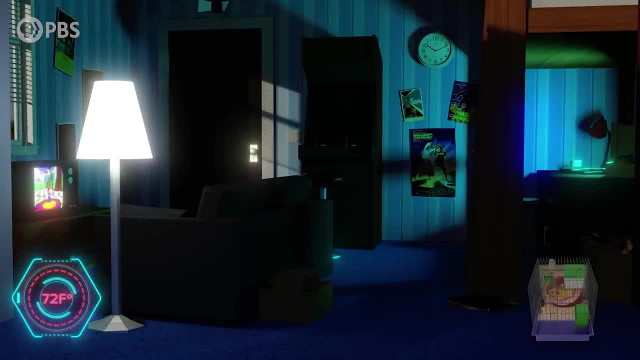 And the second law seems to be an emergent law. Emergent properties and laws arise from the statistical behavior of large numbers of particles. For example, E ты之 Land- A room full of air, has a temperature which is a measure of the average energy of motion. 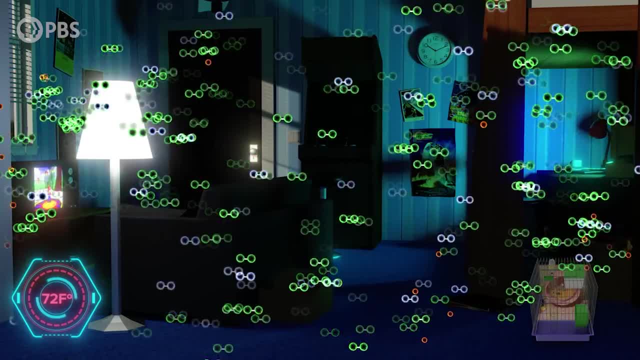 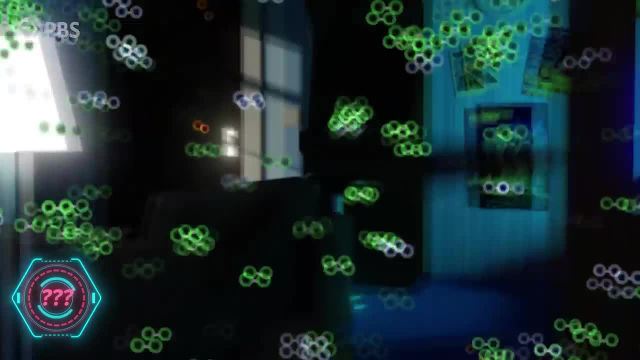 of all the individual air molecules. But a single air molecule doesn't have a temperature, at least not in the same way. Instead, that molecule has a velocity and a mass and so on, which define how it bounces off the walls or other particles, giving rise to what we perceive as temperature and giving 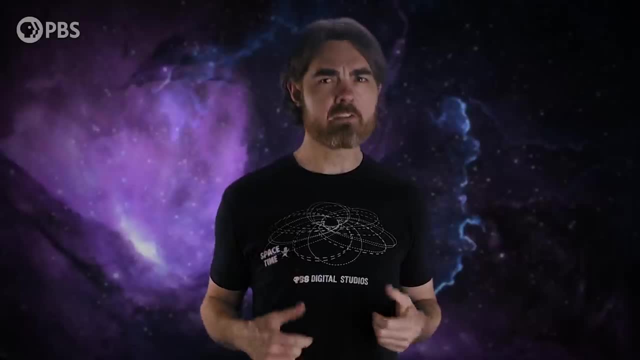 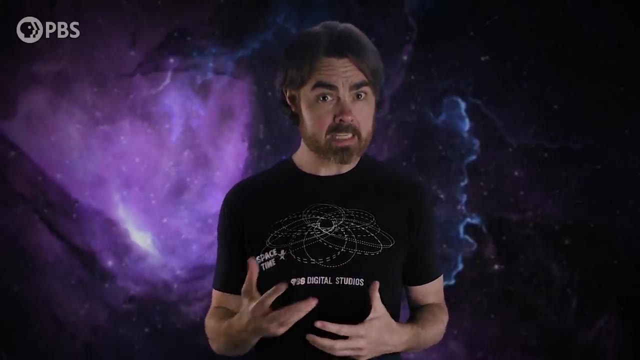 rise to the laws of thermodynamics, So we tend to think of emergent properties and laws as less fundamental than the properties and laws governing individual particles. Entropy is a thermodynamic property and the second law is well the second law of thermodynamics. 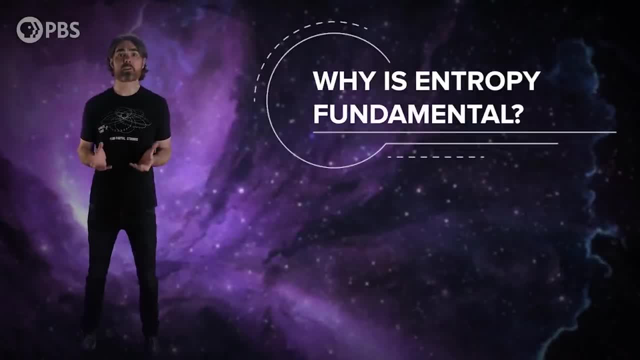 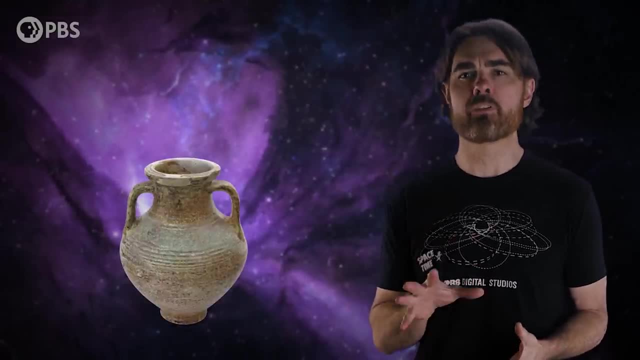 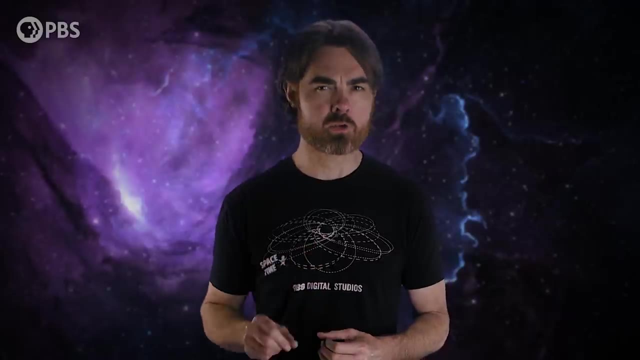 so is also statistical in nature. Why, then, are these things considered so fundamental? To answer that we need to understand what entropy and the second law emerge from. What underlying property of nature do all these different definitions of entropy describe? As is often the case, getting more fundamental means getting quantum. 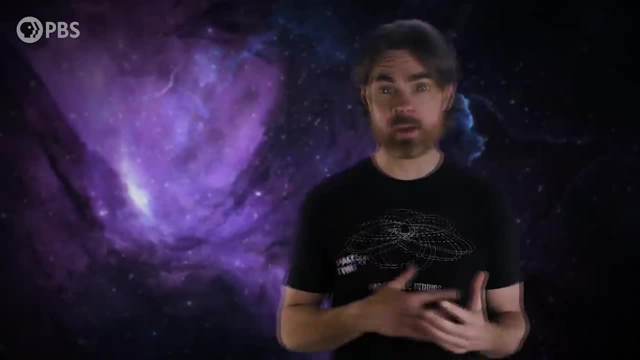 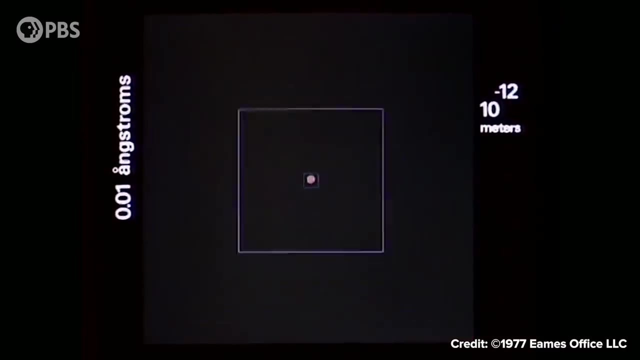 And there is indeed a type of entropy that applies to quantum systems, Just like our air molecule. it's von Neumann entropy, And understanding it may help us understand not just the second law, but also the arrow of time and how the large-scale world emerges from the quantum world in the first place. 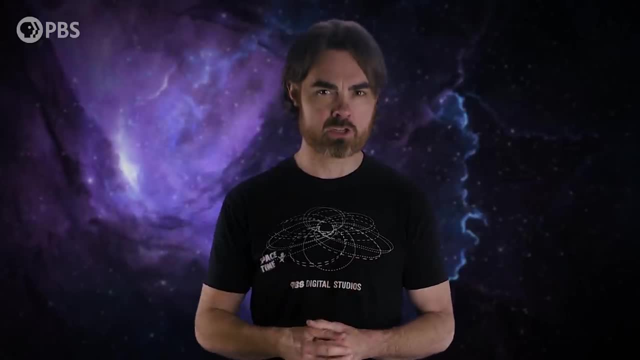 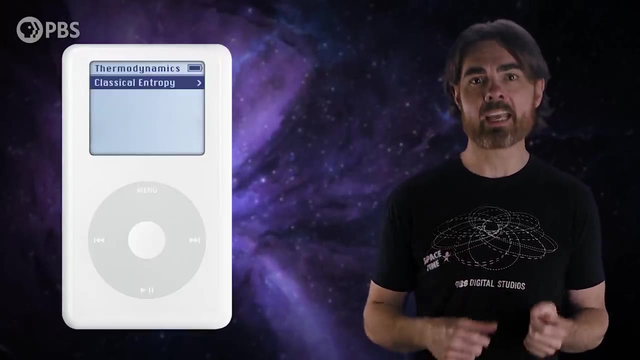 Now, before we dive into that, let's review our more familiar definitions of entropy To really understand these. we have a full playlist on the mysteries of what I'll call classical entropy and its relationship to information, But let's run through them. Rudolf Clausius came up with the first definition. 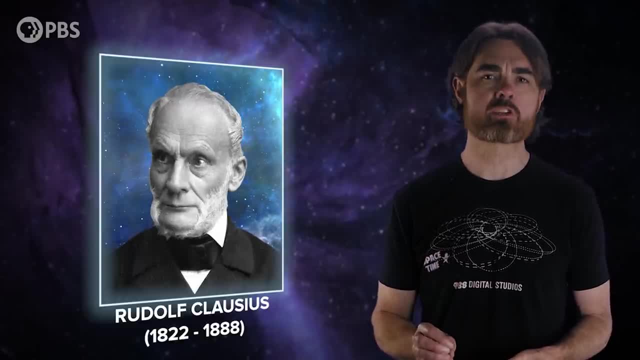 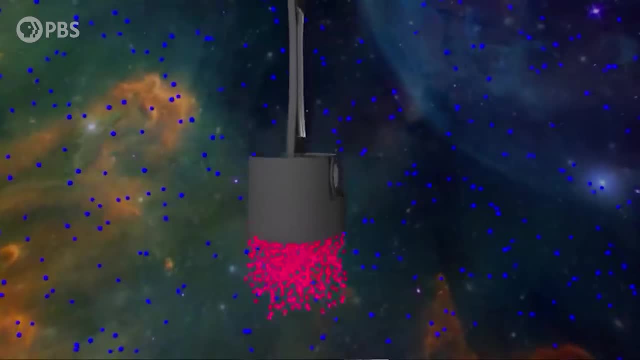 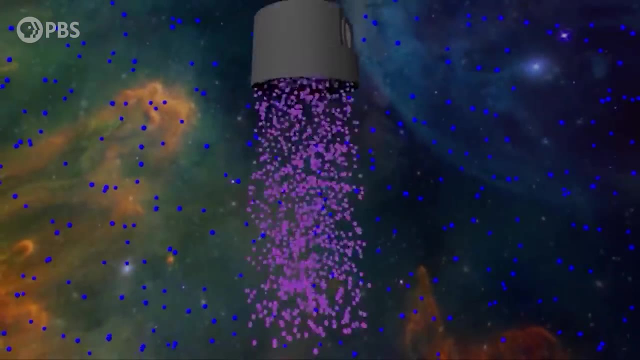 The first definition of entropy is essentially the amount of useful work that could be extracted by moving heat energy around. If heat energy is perfectly mixed inside and outside of an engine, then no work can be extracted, While if heat energy is separated hotter inside, say the piston chamber, then it will tend. 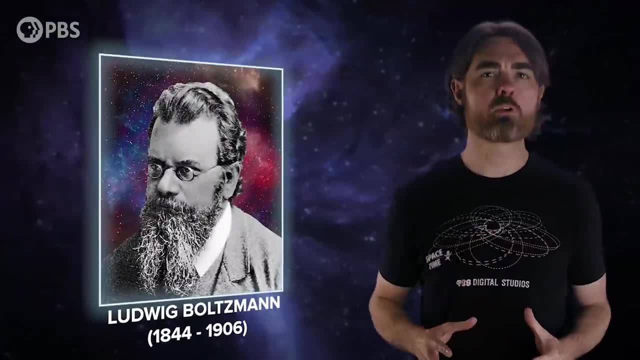 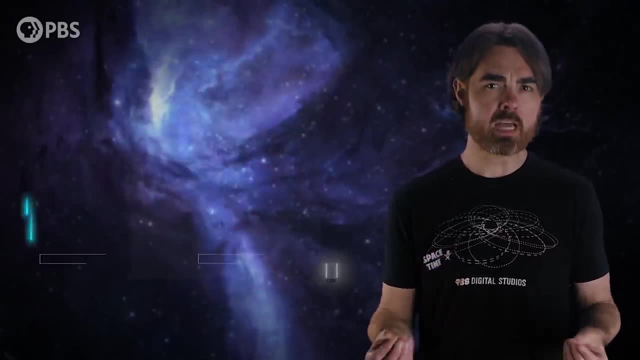 to become mixed and we can harness that flow. Ludwig Boltzmann recast entropy in terms of the number of configurations of particles that give the same set of crude thermodynamic properties. For example, There are more configurations of particles in which energy is perfectly mixed than if. 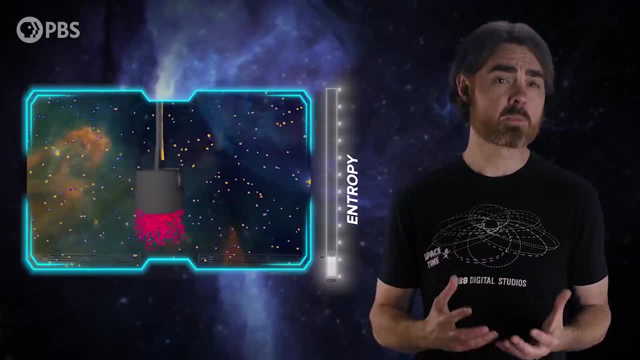 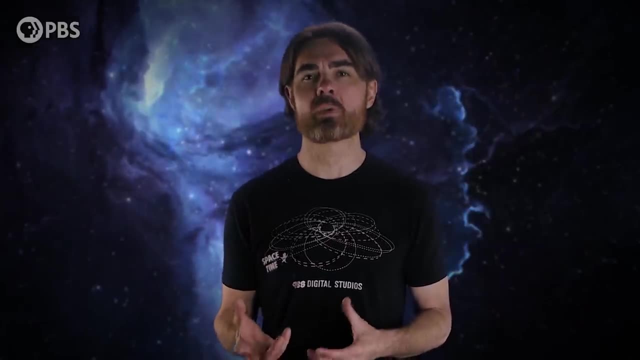 energy is concentrated in one spot, like in our piston chamber Systems, will tend towards the more common configurations, hence entropy increases. Here we start to see the connection between entropy and information. If all the air is in the corner of the room, for example, then you know more about the 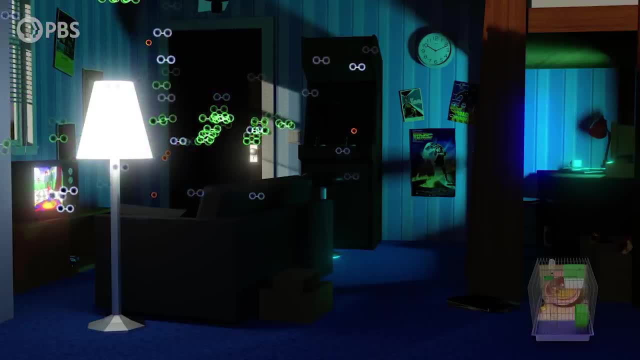 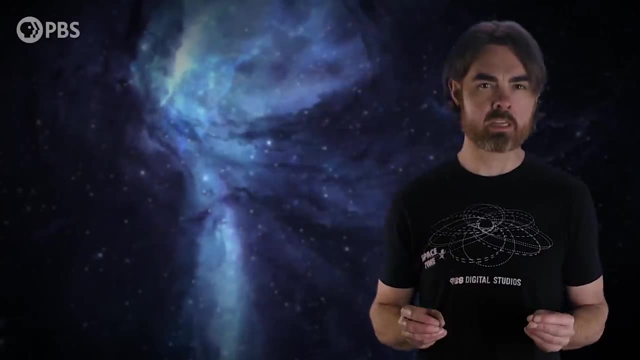 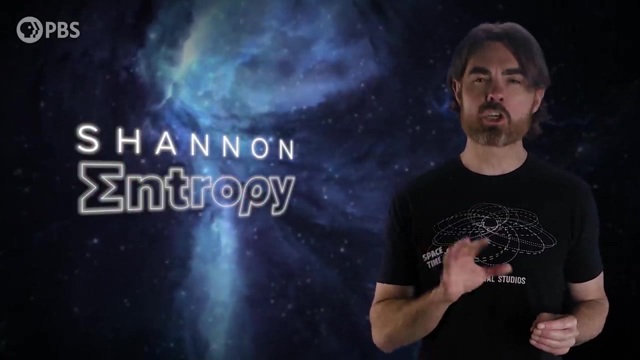 positions of the individual particles versus if they're spread through the room. But it took the invention of information theory to really see the connection between information and entropy. It was Claude Shannon who founded the field of information theory and also invented the entropy of information- Shannon entropy. 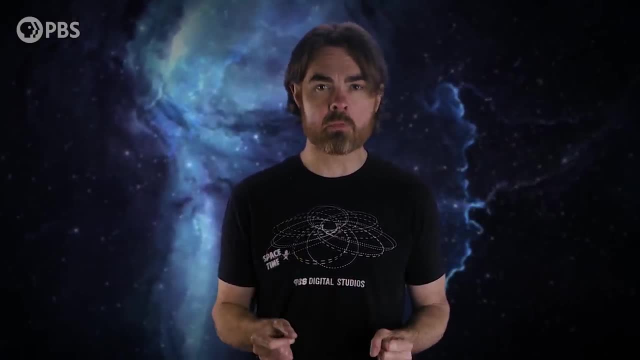 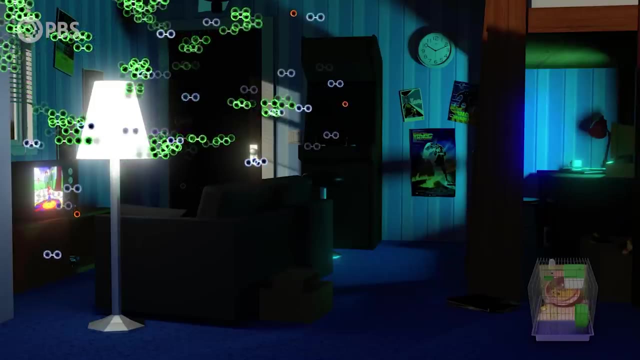 Shannon, entropy can be thought of as the amount of hidden information in a system or, more precisely, the amount of information we can hope to gain by making a measurement of the system. If all the particles are bunched up in the corner, then measuring their exact positions. 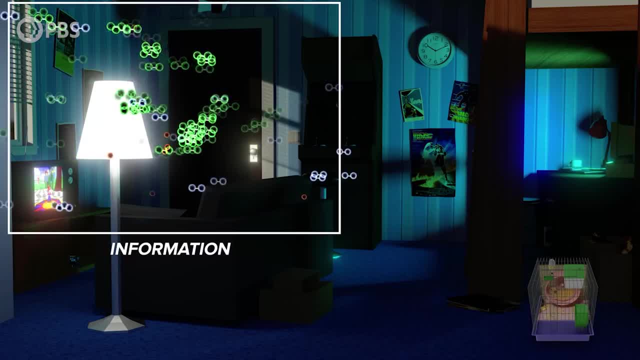 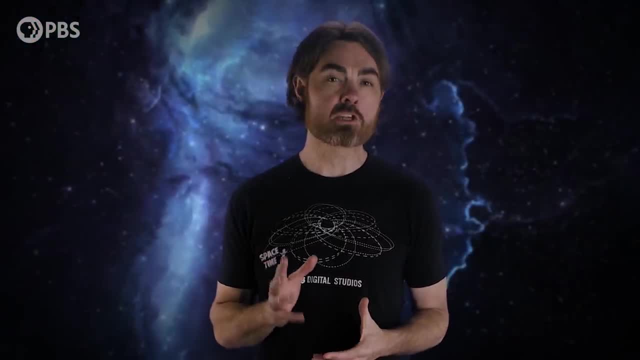 gets you some information, But if you measure the positions when they're spread through the room, you increase your information by a lot. Another way to think about Shannon entropy is in terms of events. The more possible outcomes of an event, the more entropy the event has. 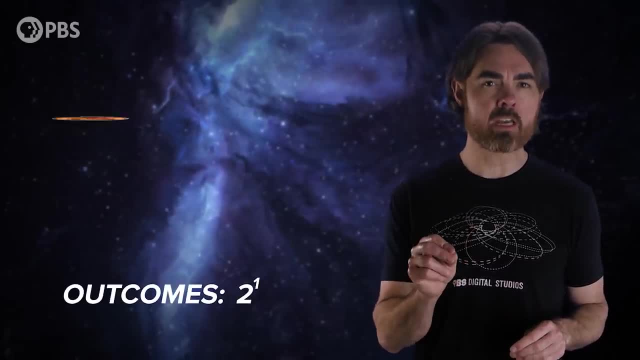 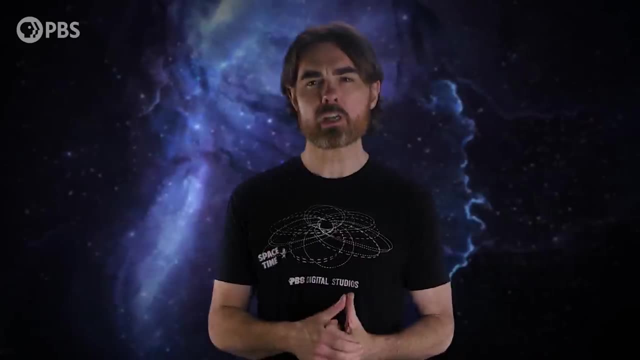 For example, a flipped coin is a low Shannon entropy event because it only has two outcomes, while flipping a million coins is a high entropy event. Shannon entropy is actually more fundamental than thermodynamic entropy in that it is a generalization of the more familiar entropy. 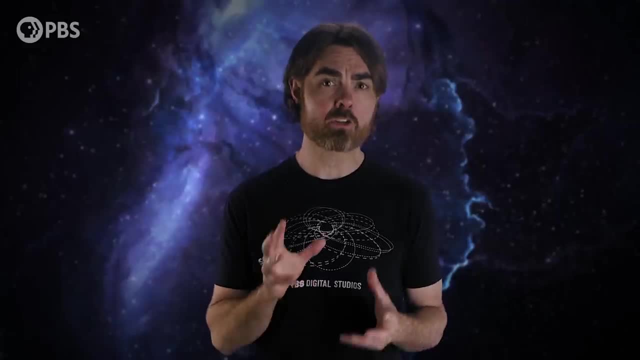 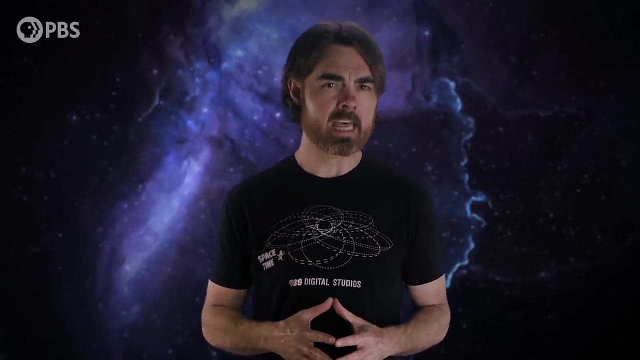 It applies to any system of information and any type of action. Shannon entropy is a generalization of the more familiar entropy. It applies to any system of information and any type of action that reveals that information. When he first came up with this theory, though, Shannon didn't fully realize its importance. 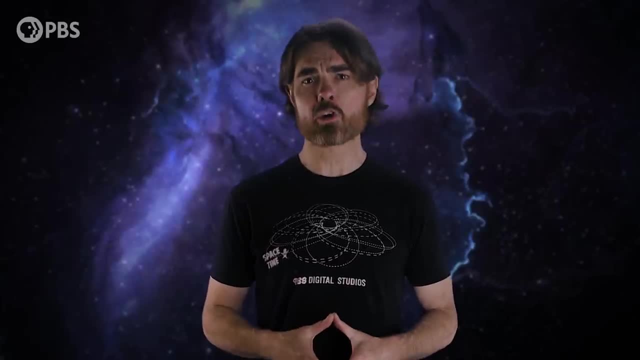 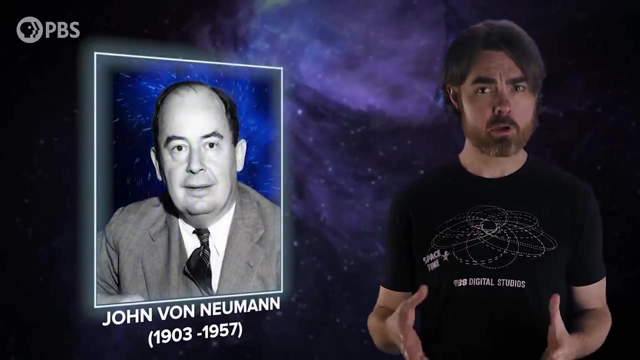 As the perhaps apocryphal origin story goes, he only started calling his invention entropy after talking to the great Hungarian mathematician and physicist John von Neumann. Supposedly von Neumann said that he should call it entropy for two reasons. 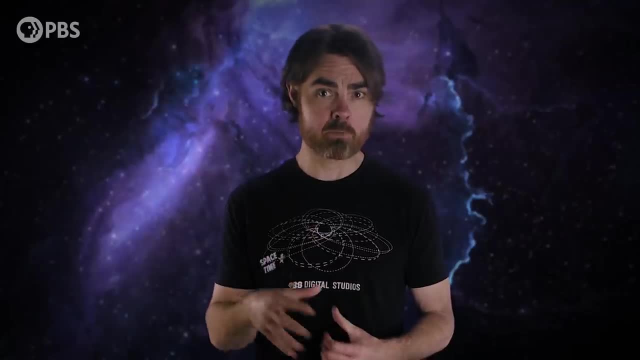 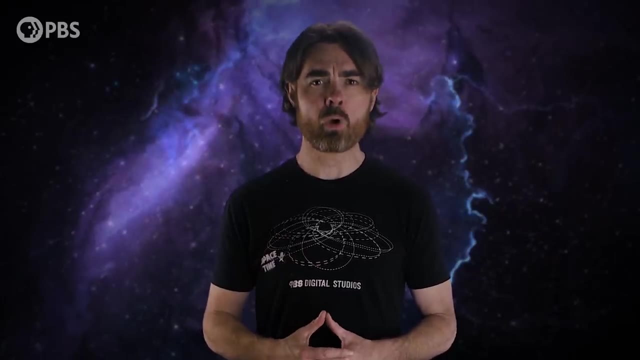 One, it looks exactly like the equation for thermodynamic entropy. and two: nobody knows what entropy is. so nobody knows what entropy is. Nobody would argue with him. But von Neumann probably knew perfectly well that Shannon's entropy was the real deal. 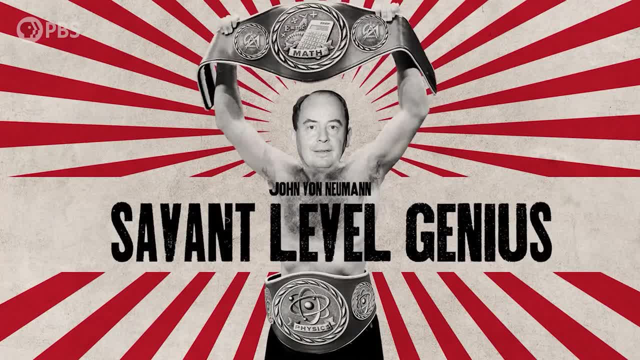 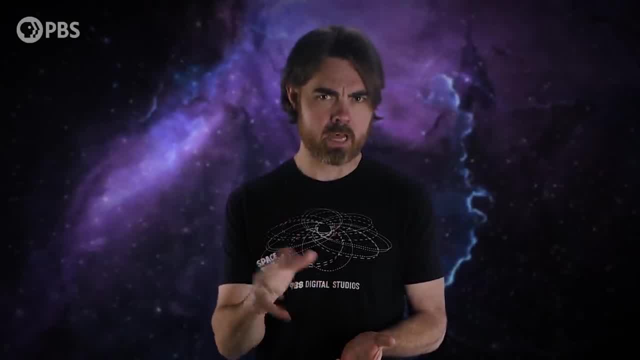 One because von Neumann was a savant-level genius who had out-mathed and out-physiqued many of the greatest minds of the last century, And two because, of part one, von Neumann had already invented his own brand of entropy. 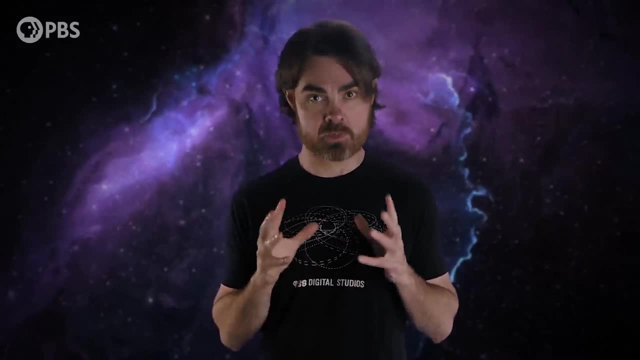 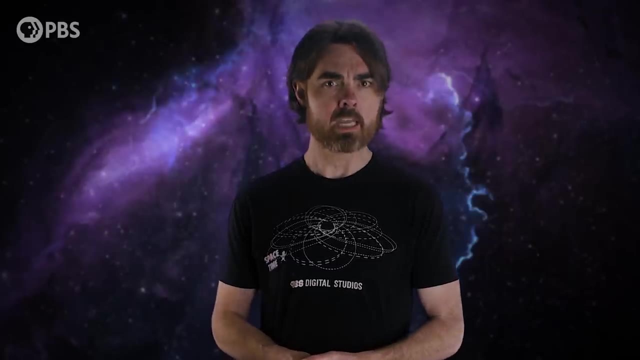 – von Neumann entropy. It's the entropy of quantum systems, And because everything else is made of quantum systems, it may be the most fundamental definition of entropy. Even Shannon entropy is just a special case of von Neumann entropy, At least so says von Neumann himself. 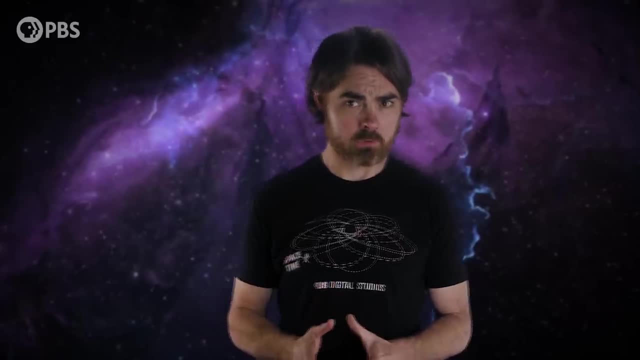 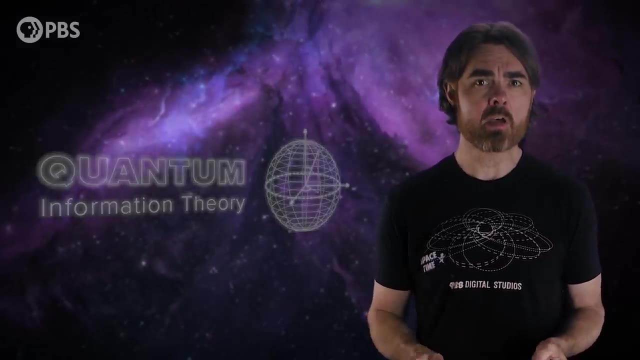 The concept of von Neumann. entropy is at least incredibly powerful. It's at the heart of quantum information theory, enabling us to calculate how much quantum information is contained in a system, and it can also be used to determine how many bits of classical information we can get out of the system when we make a measurement. 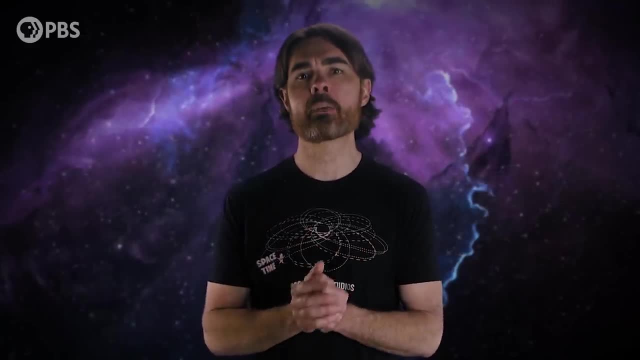 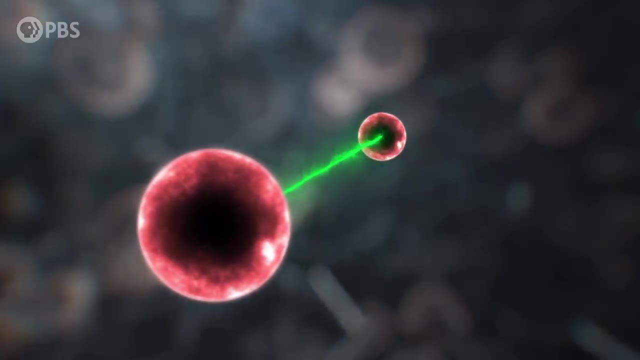 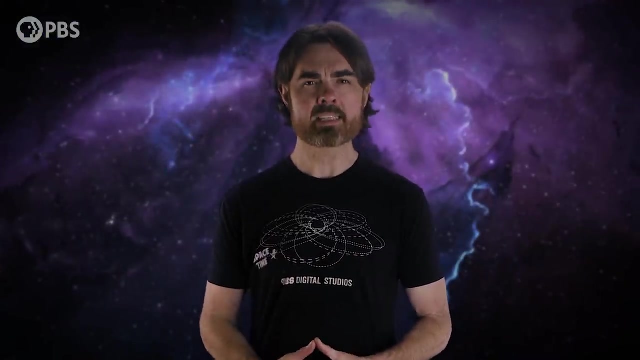 But perhaps the most interesting. von Neumann entropy tells us the amount of entanglement in a system. In fact, it's driven by entanglement – this mysterious connection between quantum particles that Einstein called spooky action at a distance. As a bit of a spoiler, von Neumann entropy seems to reveal that the evolution of entanglement 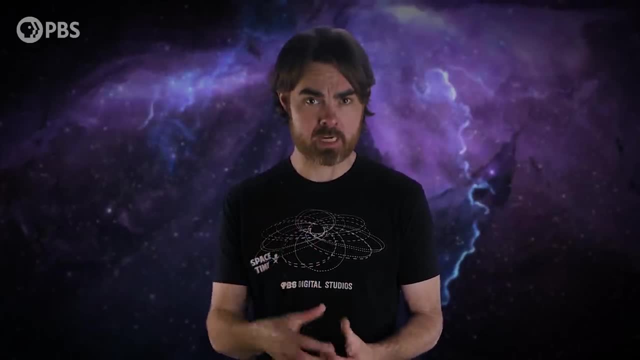 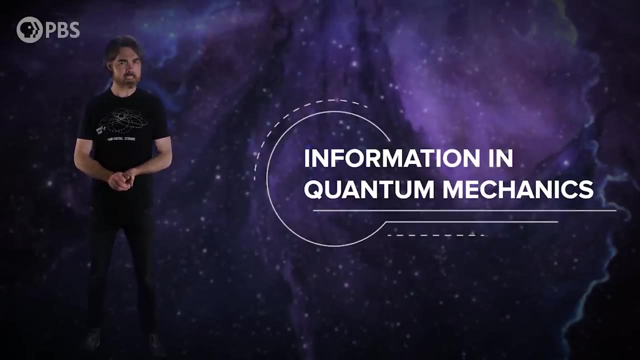 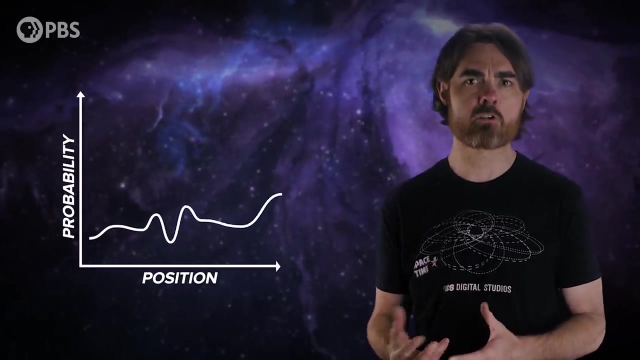 connections is what drives the second law of thermodynamics. OK, we're getting ahead of ourselves. To get a glimmer of understanding of what von Neumann entropy is about, let's think about information in quantum mechanics. Quantum systems are described by what we call the wave function – that's the distribution. 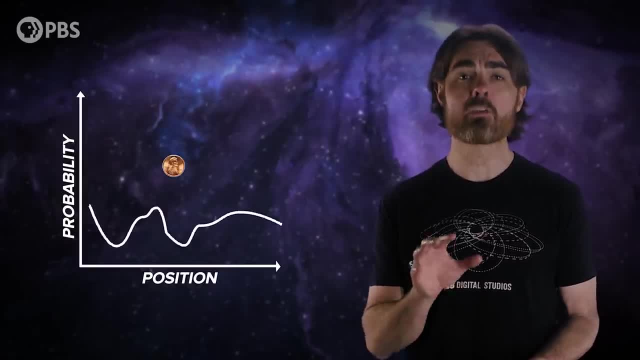 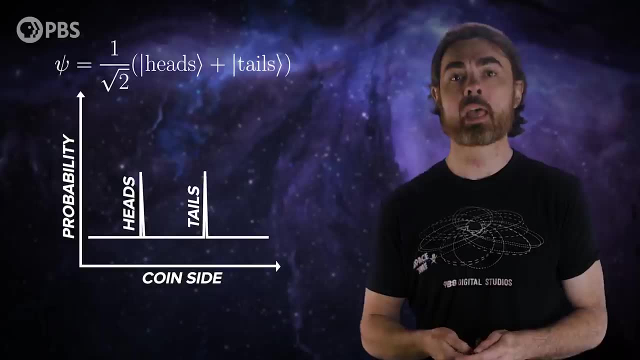 of probabilities, of all of the possible properties a system could have if you tried to measure it. As an example, imagine you have a quantum coin. It has a wave function that just describes which side is up – heads or tails. So you flip the quantum coin and it enters what we call a superposition of states. 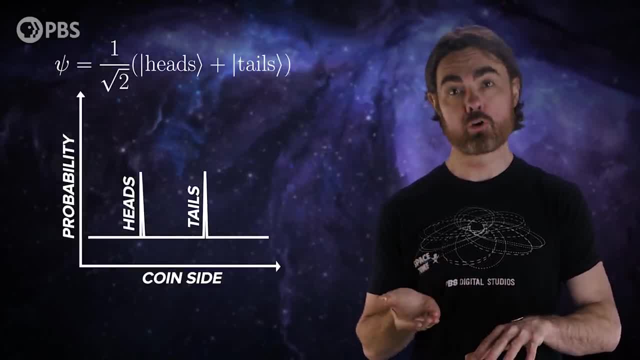 It is simultaneously heads and tails until you look at the result, at which point it becomes either heads or tails. By the way, the quantum coin is just likely both alive and dead. It's not a quantum coin. It's not a quantum coin. 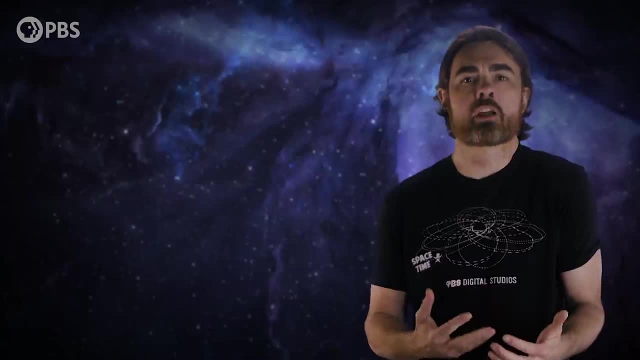 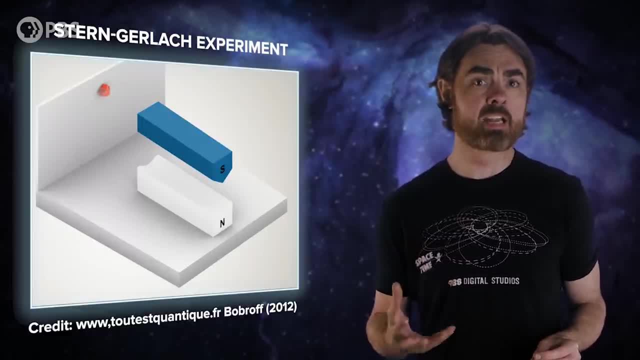 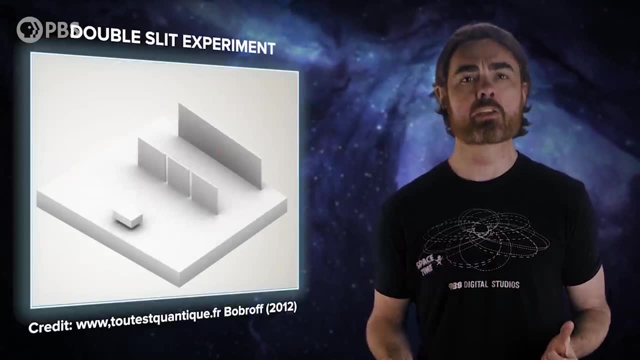 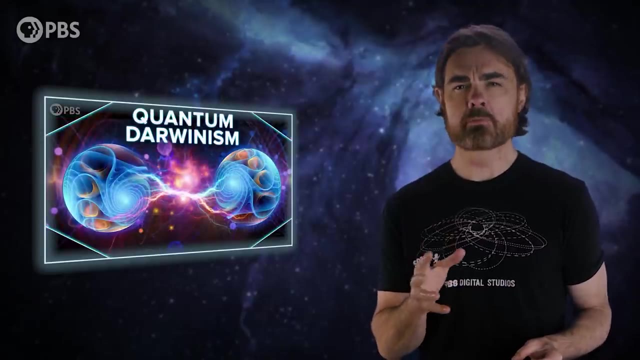 can exhibit these superposition states like a particle simultaneously having spin up and spin down, as revealed in the Stern-Gerlach experiment, or simultaneously passing through two slits in the double-slit experiment, And we've talked before about how these experiments verify these overlapping, split realities. 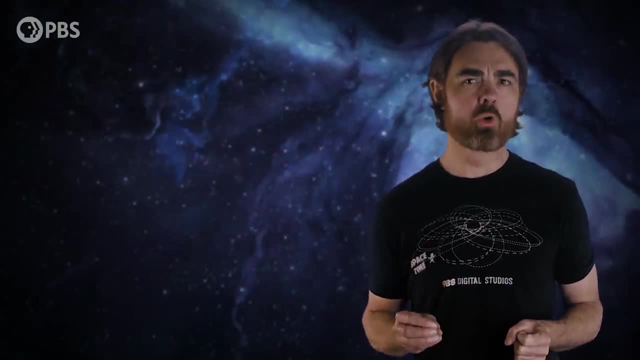 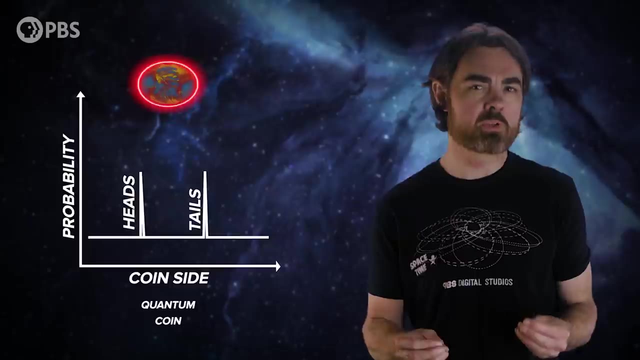 Here is a counter-intuitive thing about superposition. After you flip the quantum coin, you actually do know its current, unrevealed state. That's because its state is entirely defined by its superposition wavefunction. It is in a pure state of 50% heads and 50% tails. 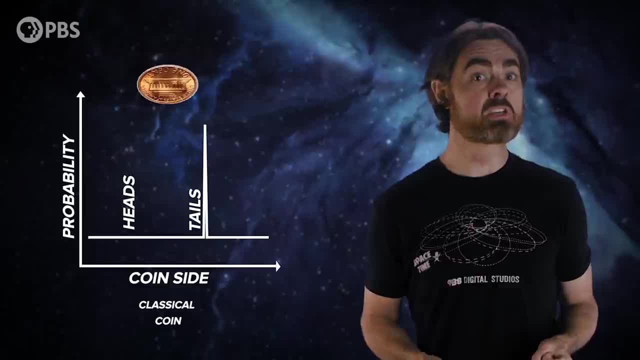 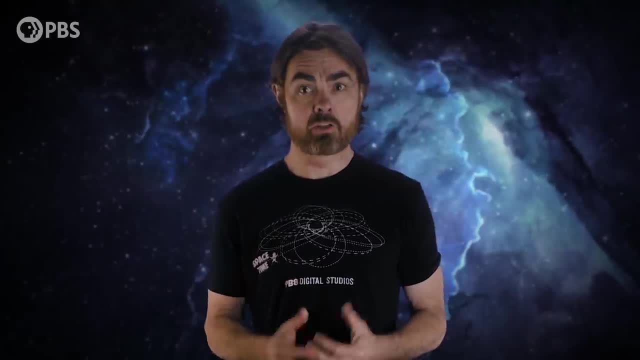 This is subtly different to the state of a classical coin, which is either heads or tails, with a 50% chance of each. That superposition really represents the coin's current reality from your perspective. But if you have full knowledge of the unrevealed state of the quantum coin, you will be able 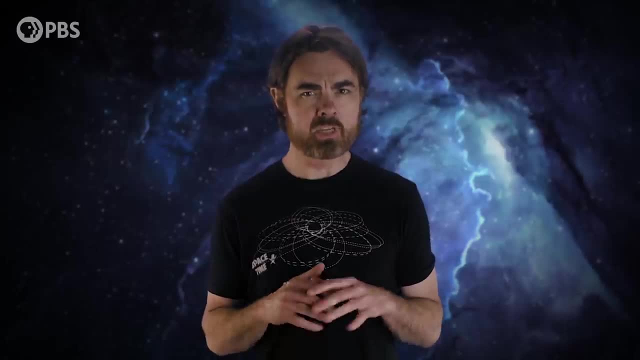 to see that the state of the quantum coin is the same as the state of a quantum coin. If the state of the quantum coin is the same as the state of a quantum coin, then there is no hidden information, which means its entropy, in this case its von Neumann entropy. is zero. Observing the coin doesn't reveal new information about that unrevealed state. rather, it changes the quantum state in a random way- now 100% heads or 100% tails. but the information about which way it would go wasn't hidden in the unrevealed wavefunction. This is very different from the result of flipping a regular coin which is entirely heads or tails before you reveal it. That information is embedded in its wavefunction. it just isn't known to you. So the regular coin's entropy, in this case its Shannon entropy, is positive. 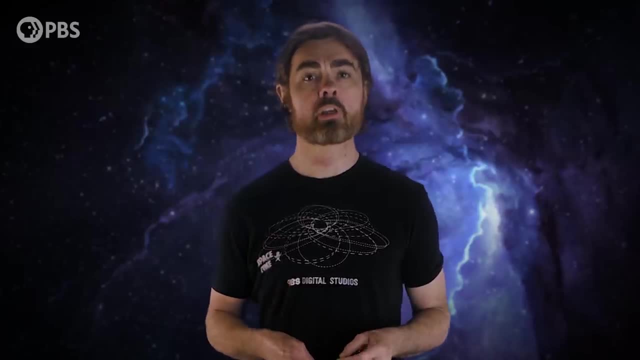 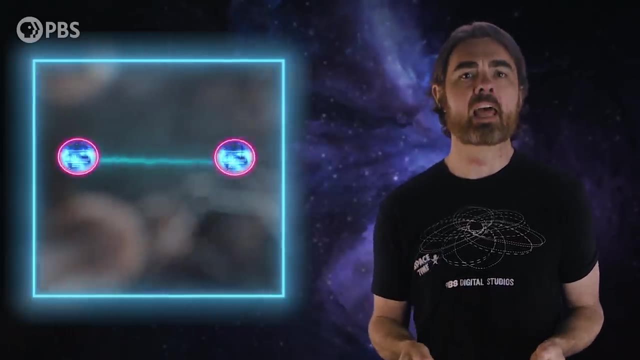 In case superposition wasn't weird enough, let's bring in quantum entanglement. That means we need a second coin. It's spookily connected to the first in that when both coins are flipped they have to land opposite to each other. 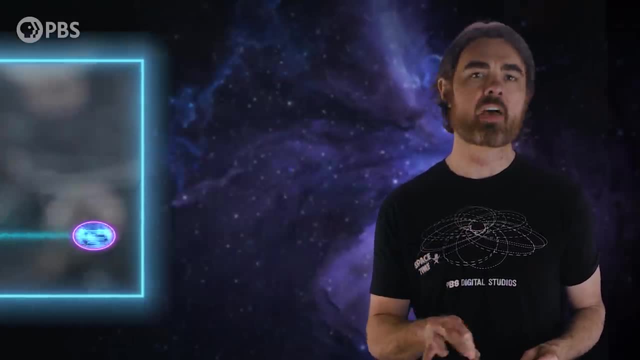 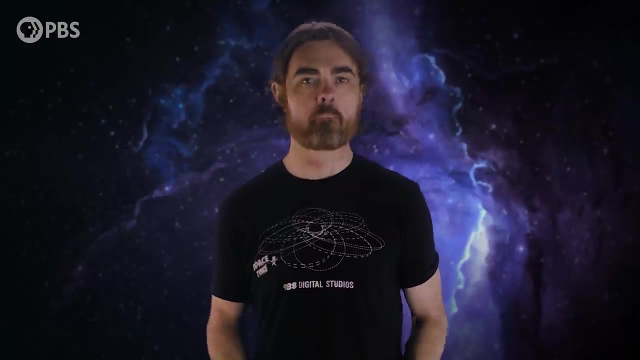 After the flip: we say that the flip results are entangled, They are correlated. Even though we don't know the individual results, if we reveal one we'll immediately know the result of the other. So you flip your pair of entangled quantum coins. 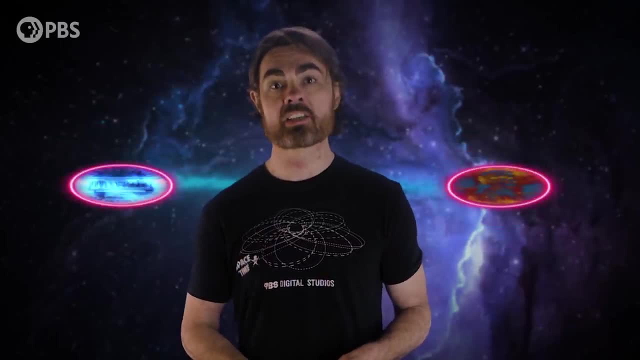 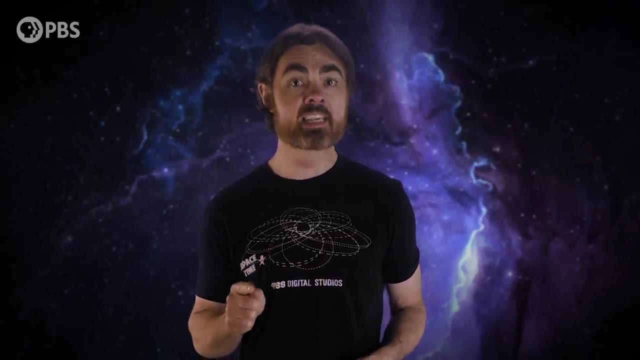 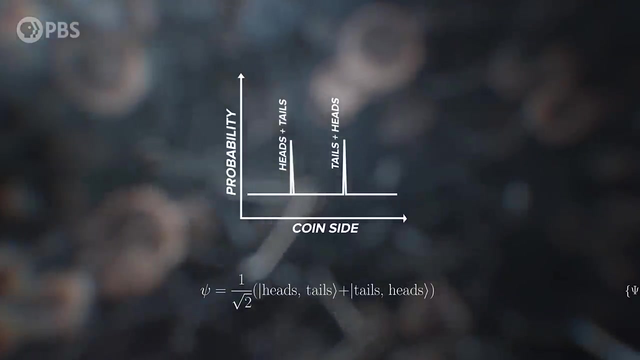 There are two ways they can turn out. Either the first coin lands tails and the second heads, or vice versa. Before they're revealed, they exist in a superposition of states. Both possibilities exist simultaneously. The unrevealed wavefunction is like this, which means 50% heads- tails and 50% tails- heads. 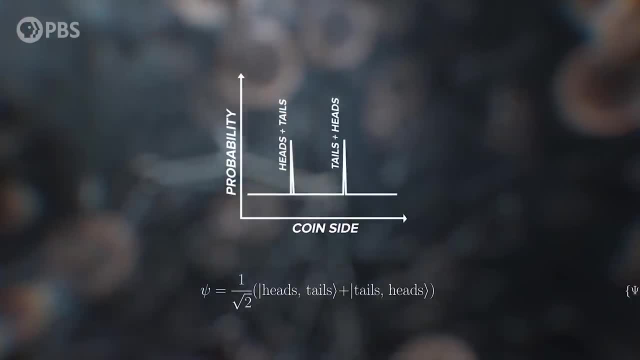 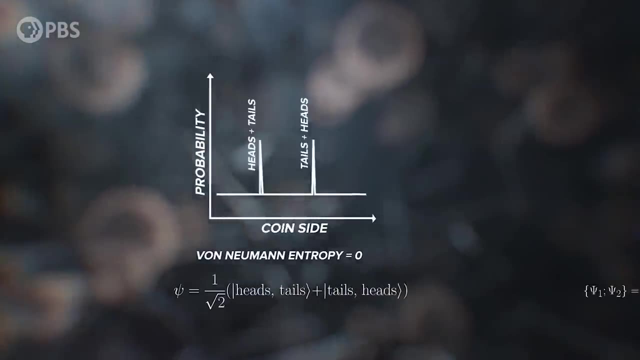 The von Neumann entropy of that entire wavefunction is still zero because the combined wavefunction of the two coins holds all the information about their current state. But what if we consider only a single coin, Because of the entanglement, the part of the wavefunction corresponding to a single coin? 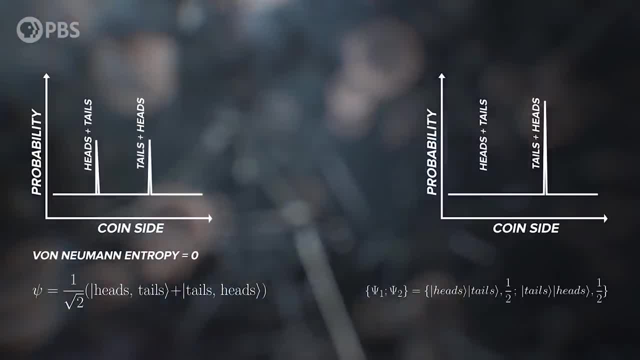 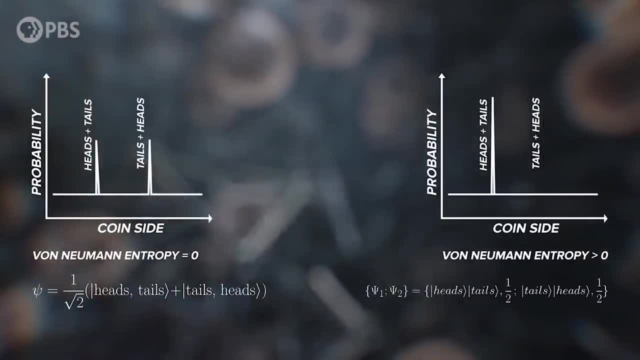 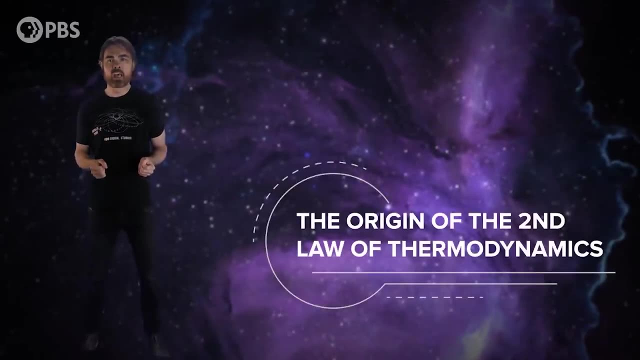 does not contain all the information about the coin's state, Its. von Neumann entropy is no longer zero. Information IS hidden. It's hidden in the part of the wavefunction corresponding to its entangled partner. That's it, And this is where we can connect von Neumann entropy to all of the other forms of entropy. 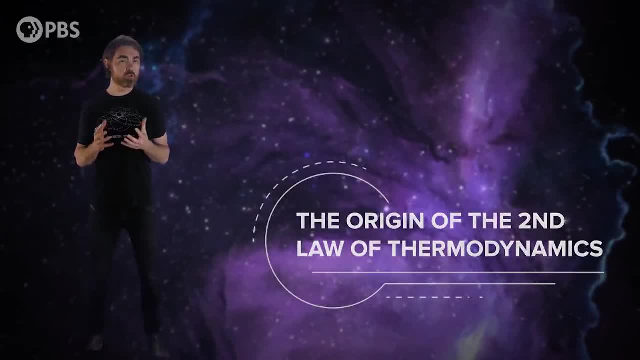 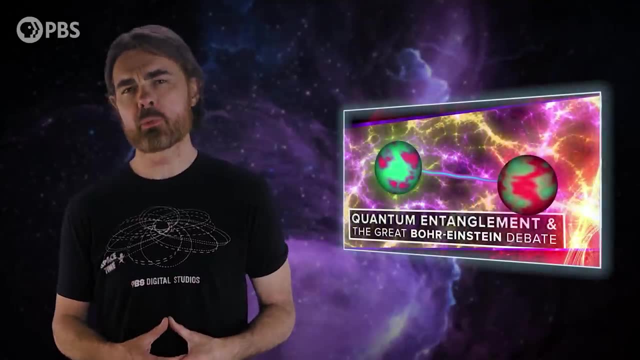 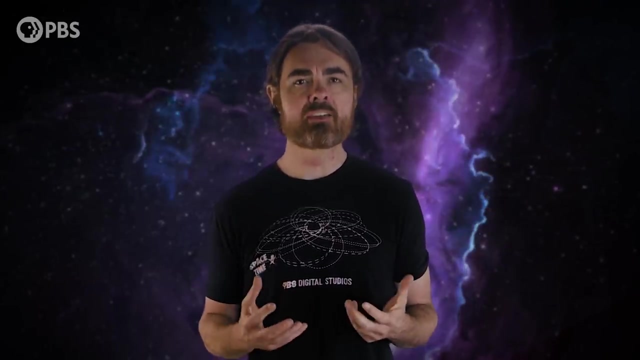 and glimpse the real origin of the second law. When viewed with its entangled partner, the coin exhibits quantum weirdness, like superposition, that could be revealed in experiments like a Bell test, which we covered previously. But treated individually. each separate entangled quantum coin behaves kind of like a regular classical coin. 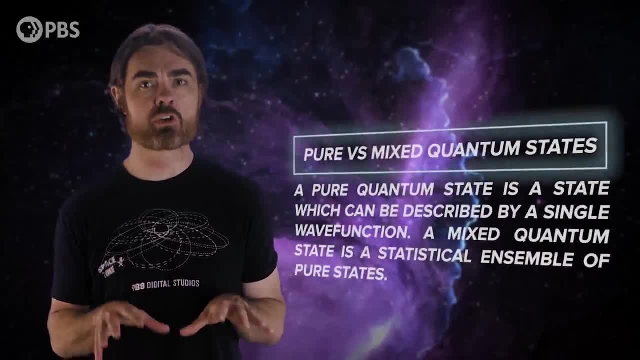 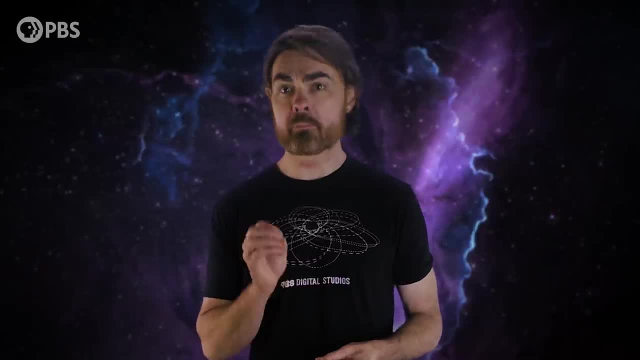 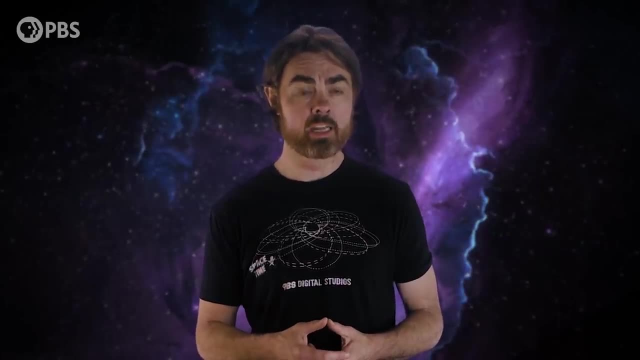 For example, it doesn't by itself exist in a pure superposition of states. That superposition only appears when you include its entangled partner. It's in what we call a mixed state- heads or tails, not heads and tails- And just like the regular classical coin, it has non-zero entropy. 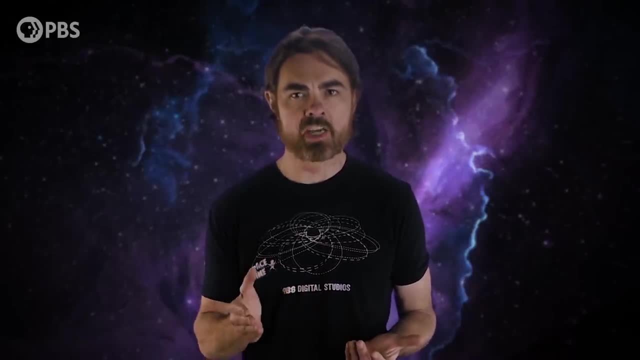 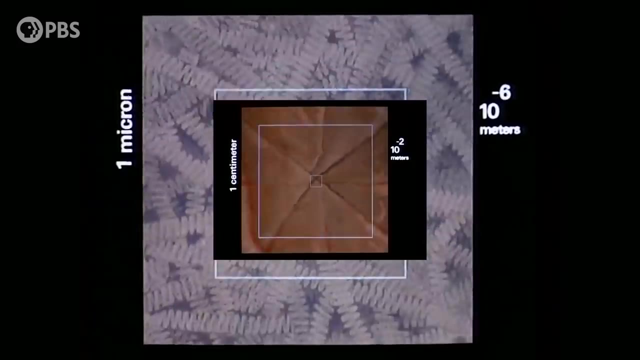 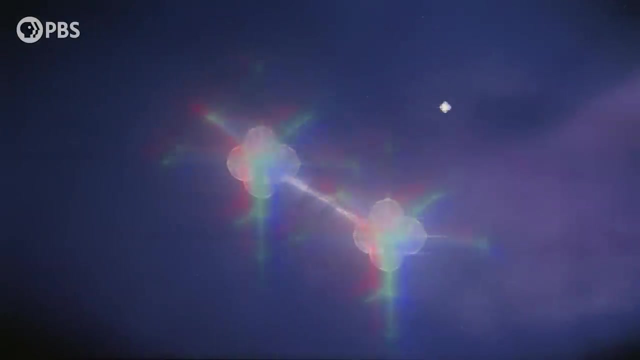 This similarity between the classical coin and the entangled but isolated quantum coin is no coincidence. Its entanglement is the first step in the transition between the quantum and the classical world. Our capacity to observe quantum effects, like superposition, depends on being able to access the entire wave function. 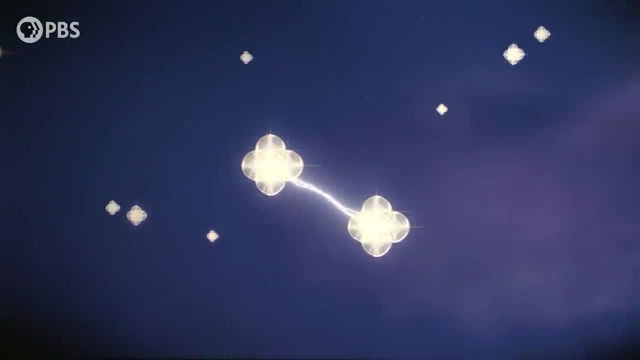 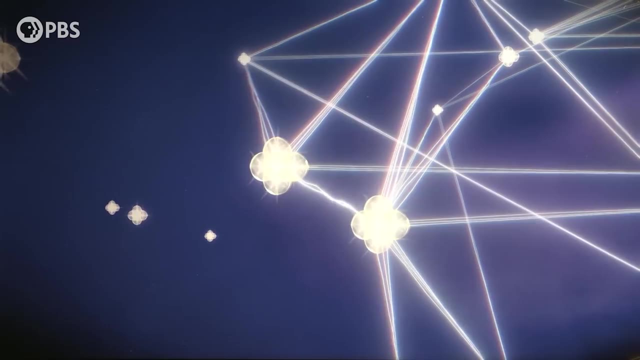 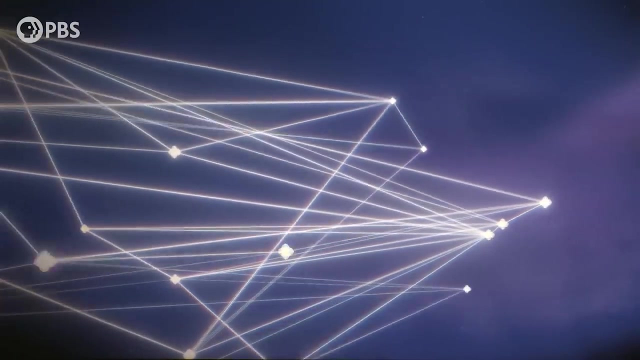 With one partner coin in entanglement that becomes more difficult. But as a quantum object interacts with the countless particles of a macroscopic environment and those particles interact with each other, the web of entanglement grows so quickly that it soon becomes impossible to access the entire wave function. 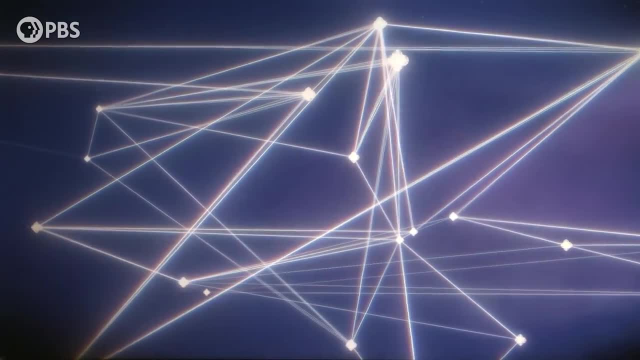 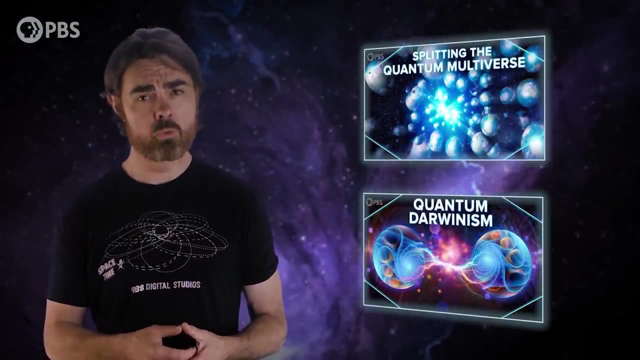 We call this process decoherence. It's how the ordinary macroscopic world emerges from its very weird quantum world. And for a deeper dive into decoherence, we do have you covered. Looking at it this way, our classical coin is just like our isolated, entangled coin. 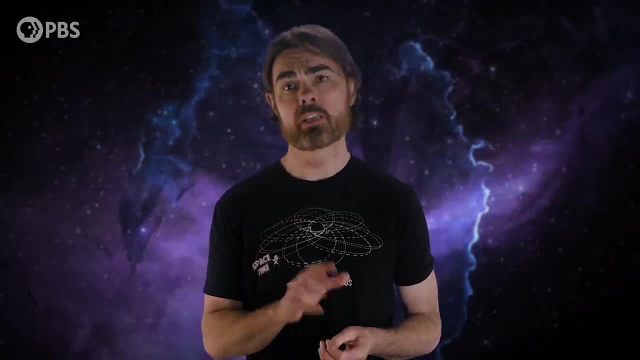 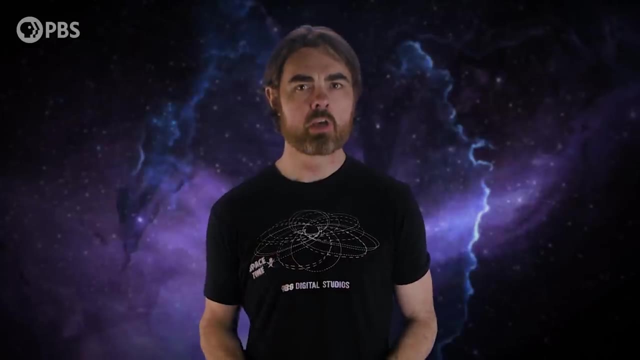 Except now we don't have a simple entanglement between two coins. The entanglement is between the coin's countless constituent quantum parts and every particle they've ever interacted with. That network of entanglement is in the superposition of states, heads and tails. 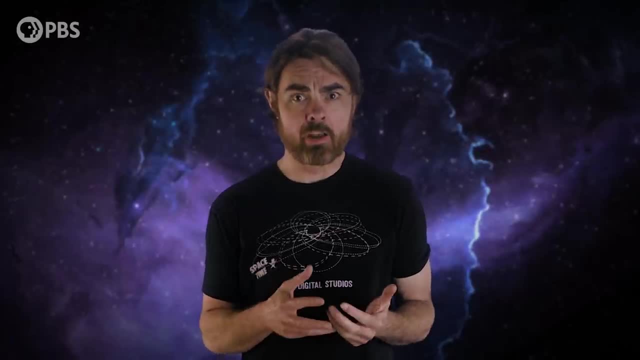 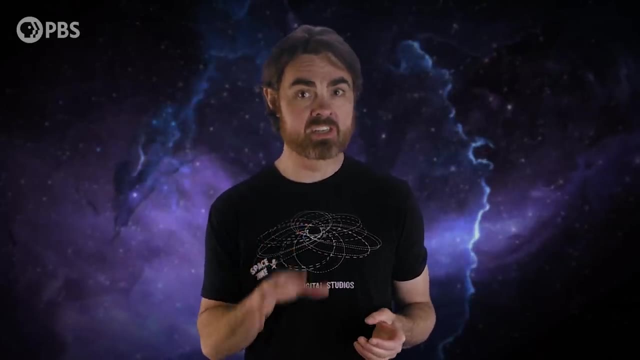 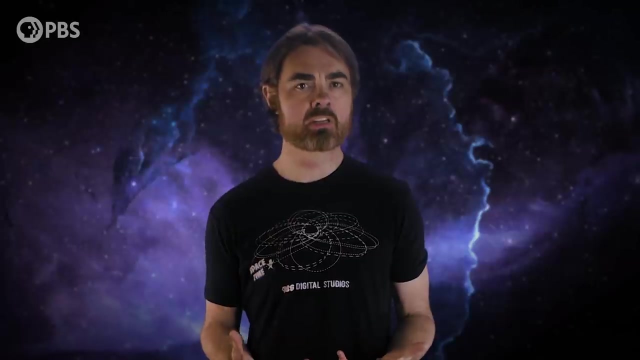 But you can't ever access it In part, because you're part of that network. you've already become entangled with the coin and live in the slice of the wave function, the mixed state where the coin is either heads or tails. The propagation of entanglement leads to our experience of the very unquantum, macroscopic world. 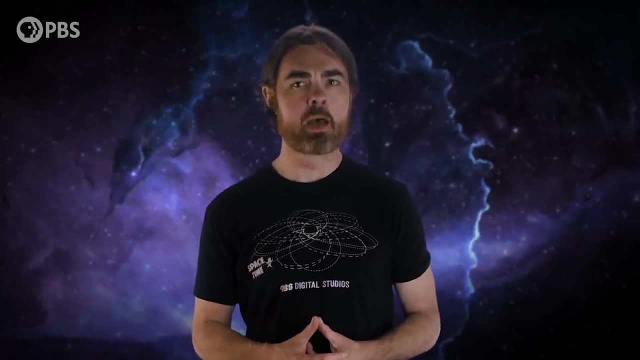 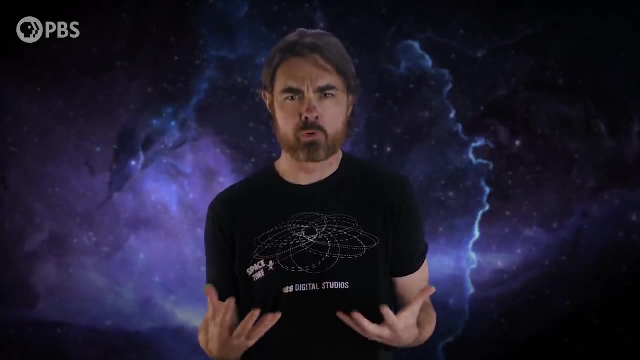 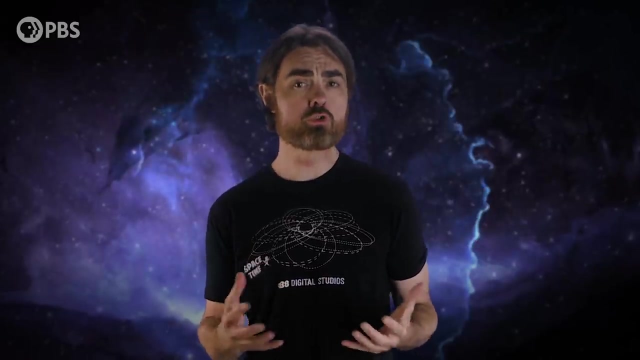 but it also drives the growth of entropy. Information about the detailed quantum states of all the particles becomes increasingly inaccessible, leaving only crude observable properties, For example thermodynamic properties like temperature. We call these properties that are preserved through this diffusion of entanglement. pointer states. 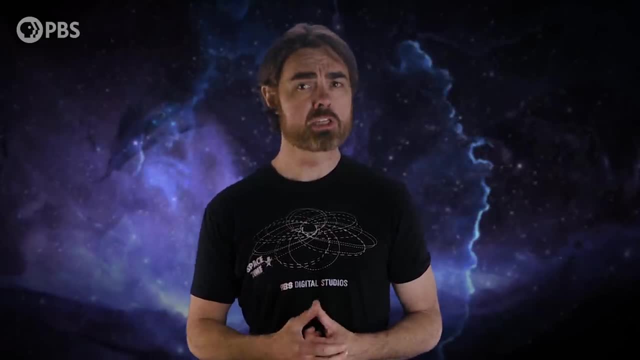 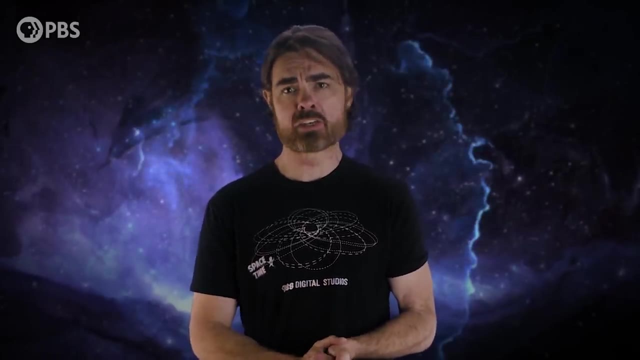 in the language of quantum Darwinism. Over time, systems move towards a state of maximum entanglement, at which point most information is hidden and the systems are describable by the fewest properties, For example, when a system equalizes to a single temperature. 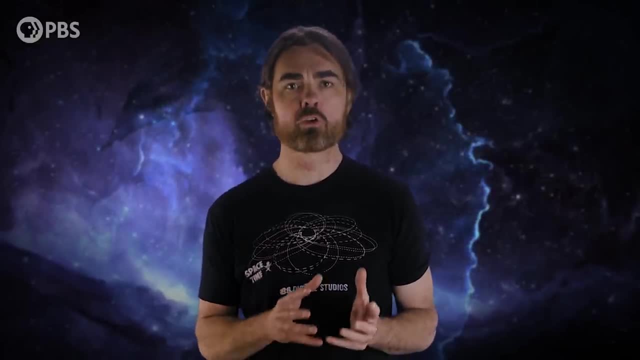 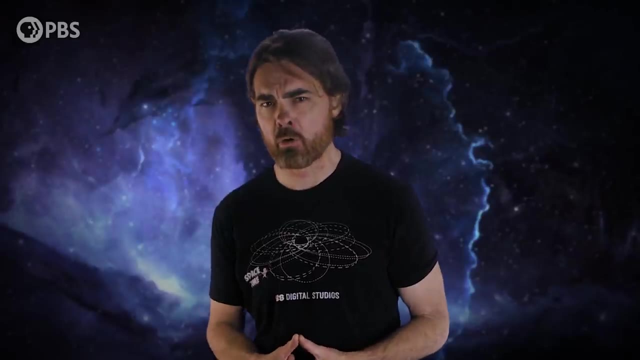 So there you have it. Growth of entanglement drives both the second law of thermodynamics and the second law of thermodynamics and the emergence of the classical world from the quantum. And, as an extra trick, it also defines the arrow of time. 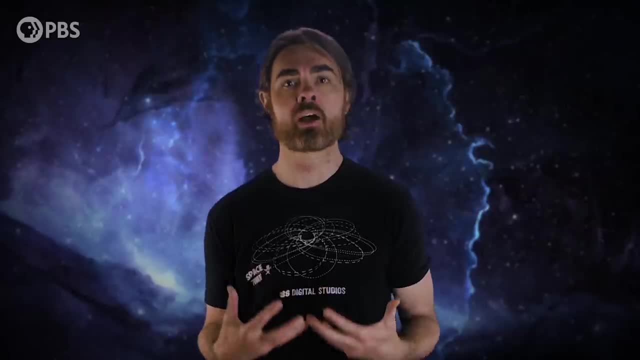 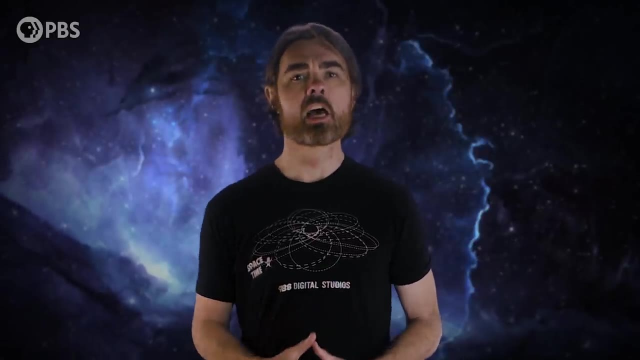 which itself points in the direction of increasing entropy and multiplying entanglement, as of course we've discussed. But there's a lot more to talk about, because von Neumann's insights lead us to a picture of reality that is more informational than physical. 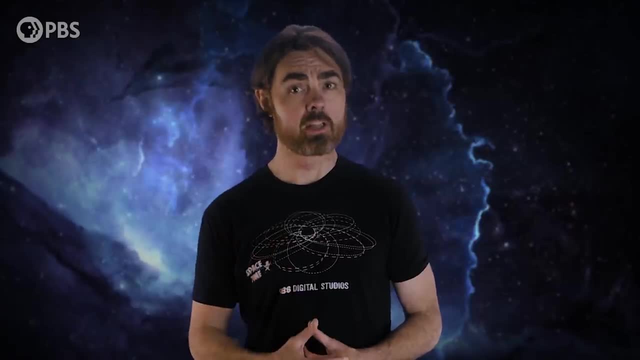 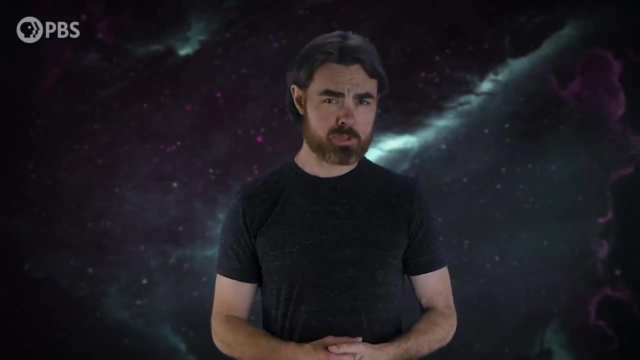 But that information won't stay hidden for long. only until our next episode of this information theorist, Space Time. Today we're doing comment responses for the last two episodes. There was the one on the Kessler syndrome, the exponential build-up of space junk around the Earth. 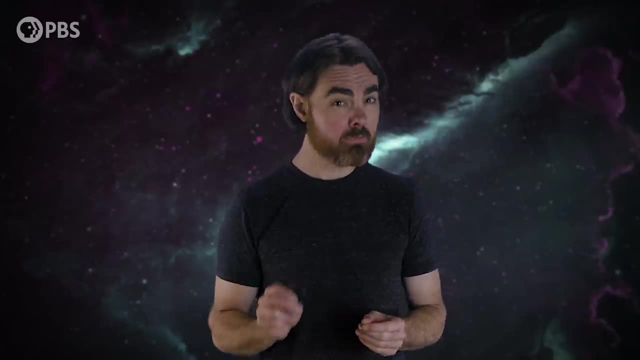 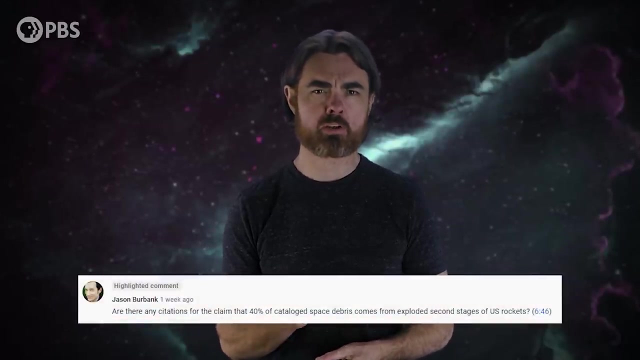 and then the one on the Planck length- the smallest meaningful length, and what that tells us about the nature of space. Jason Burbank asked for a citation for my statement that 40% of catalogued space debris comes from exploded US rocket stages. 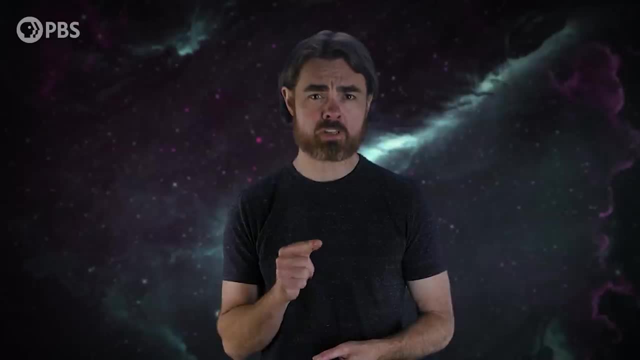 Well, I'm glad you asked, because digging up that reference and rereading it, I realize the number of times I've said that. Well, I'm glad you asked, because digging up that reference and rereading it, I realize the number of times I've said that. 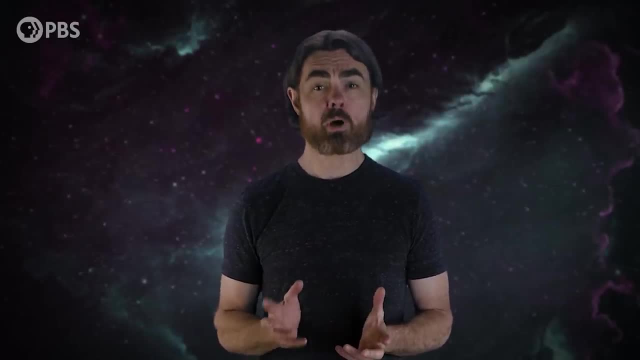 Well, I'm glad you asked because digging up that reference and rereading it, I realize the number of times I've said that The original reference is a paper by Donald Kessler back in 1981, where he finds that 42% of the debris tracked by NORAD was from 19 US rocket stages that exploded after releasing their payloads. 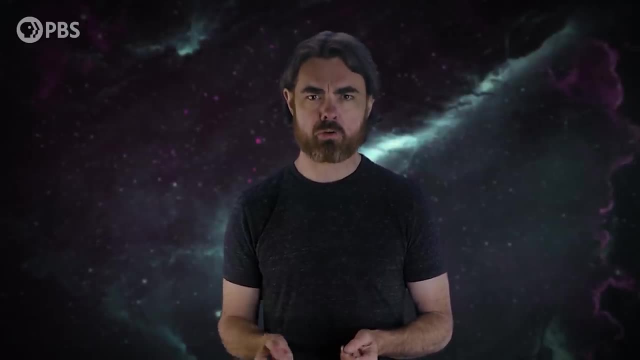 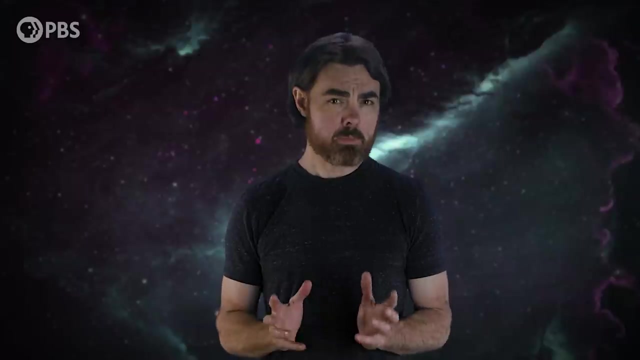 in some cases a few years later. But that was 40 years ago and the number of tracked orbital debris has increased from around 4,500 to more like 15,000.. Now, some of those new pieces were presumably due to collisions with those rocket fragments. 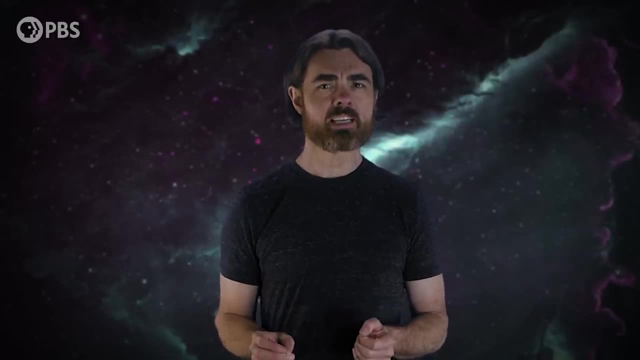 but the 42% is no longer accurate. Presumably it's lower by a factor of more than 3 due to all the new debris and the fact that some of the rocket stage debris orbits would have decayed by now. But that still leaves it at a significant fraction, just not 40%. 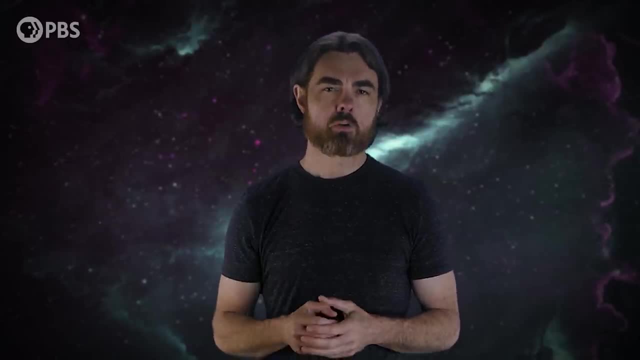 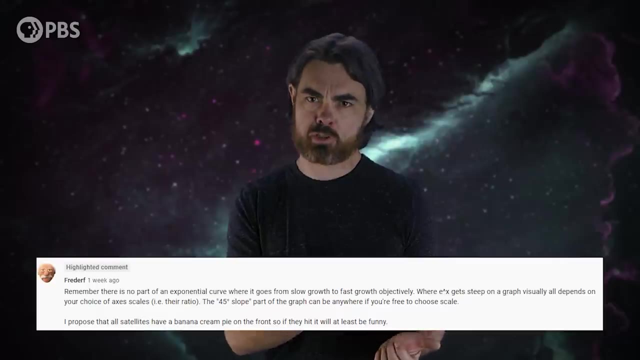 Anyway, the link to the Kessler paper is in the description Regarding exponential processes in general. Freddow reminds us that there's no part of the exponential curve that suddenly switches from slow growth to fast growth objectively, And that's exactly right. 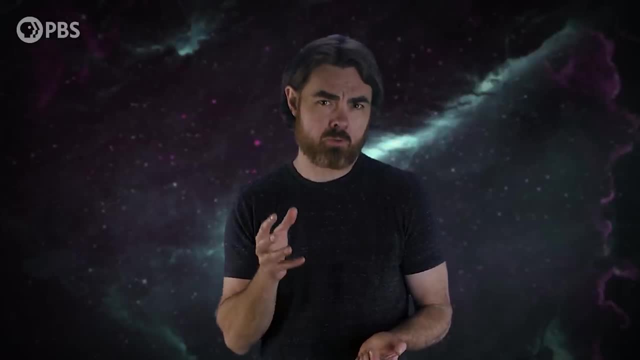 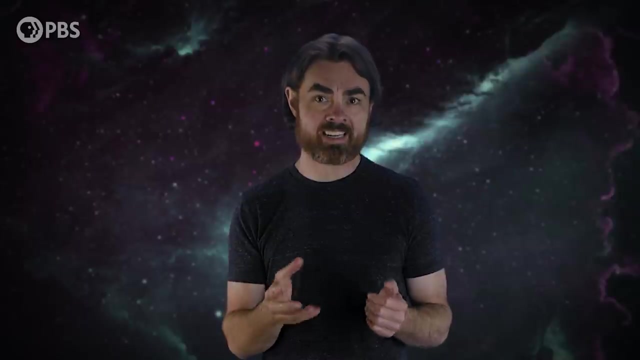 The location of the apparent kink in the curve, where it seems to go rapidly vertical, depends on the axis choice. If you zoom in on that kink, you'll see what An exponential curve. Zoom in again. Exponential curve. The exponential is scale-invariant and the location of the spot where the gradient exceeds 45% depends on the range you choose for the x-axis. 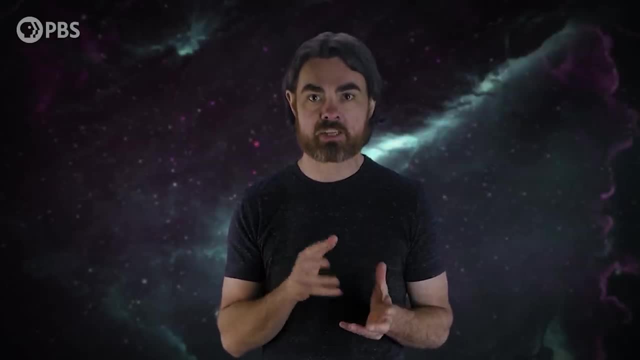 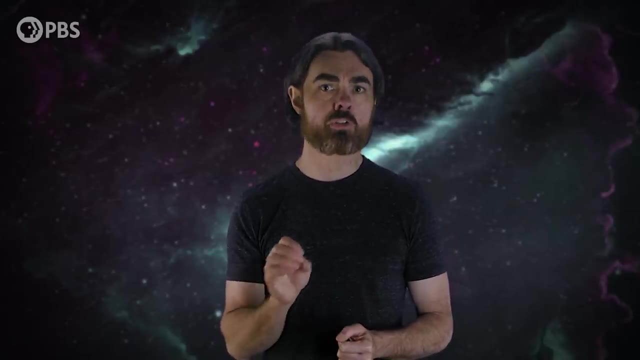 For an exponential process, the rate of doubling stays constant. Of course, the rate of doubling doesn't have to stay constant, and that may be defined by certain thresholds on the exponential rise. For example, there's a threshold in the exponential increase of space debris. 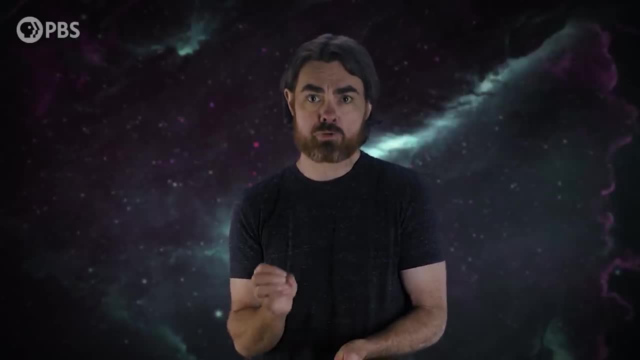 where we can no longer operate safely in space, which may reduce the rate of increase, And there's a threshold in the exponential increase of computing power, where computers are designing better computers themselves, which may actually increase the rate of increase, which may actually increase the rate of increase. 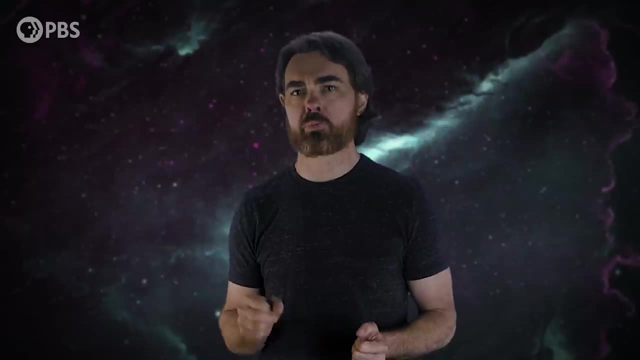 doubling rate. And then there's the feedback between exponential processes, For example. presumably our future AI overlords will be better at managing our orbital space, which will further reduce the Kessler syndrome. OK, moving on to our episode on the Planck length. 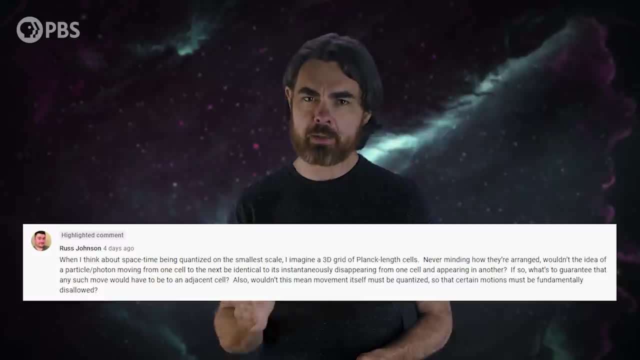 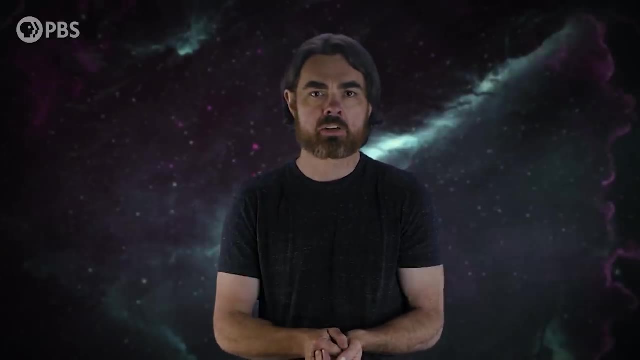 Russ Johnson asks a good one. If space is like a 3D grid of Planck length scales and movement means flicking from one cell to the next, then, a- why is movement restricted only to adjacent cells? and b- in such quantized motion would certain types of motion be disallowed? 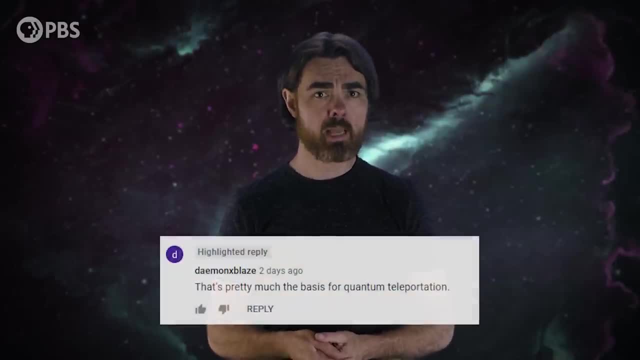 Some of you actually replied with good answers. Damon X Blaze points out that quantum teleportation, aka quantum tunneling, is basically moving instantaneously beyond your adjacent grid points. But really we can't think of space as a simple rectilinear grid. 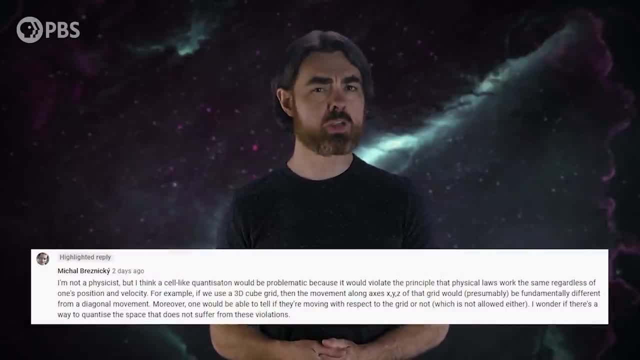 For example, Mikhail Bezniky points out that a grid like that would introduce weird effects that depend on orientation. Diagonal motion would be different from rectilinear motion. There would be preferred direction, But we know for sure that the universe has a continuous rotational symmetry. 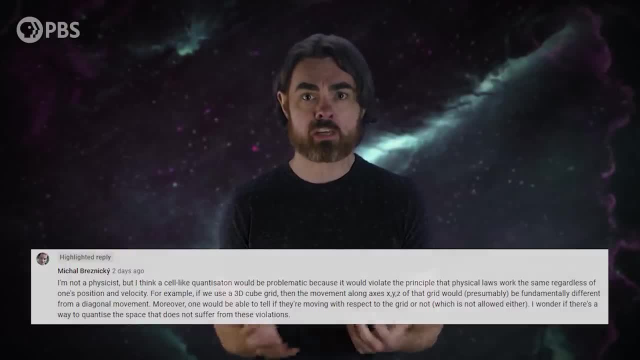 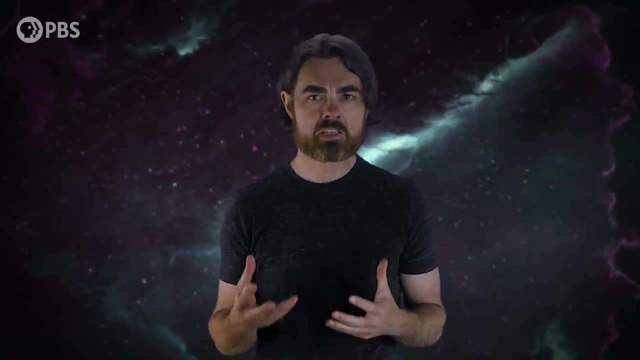 There is no preferred angle. That's the basis for the conservation of angular momentum, which we know is obeyed. Another issue is the simple grid is not Lorentz invariant? The distances have to depend on the velocity of the observer. Moving fast should then collapse the grid in one direction, but that would reduce the 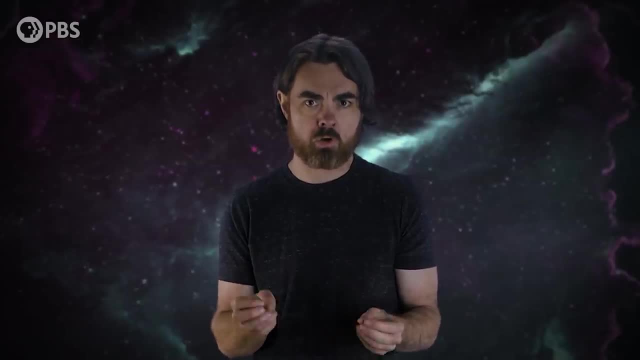 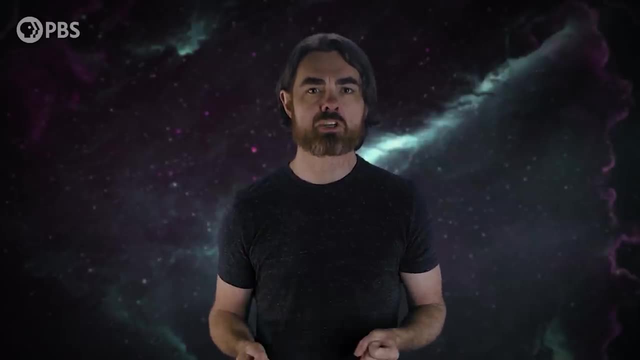 The observed Planck length should be indirect. That would reduce the grid width and hence the Planck length in that direction. Mikhail asks whether there's a way to quantize space that doesn't lead to these violations, And the answer is yes, and various people have tried. 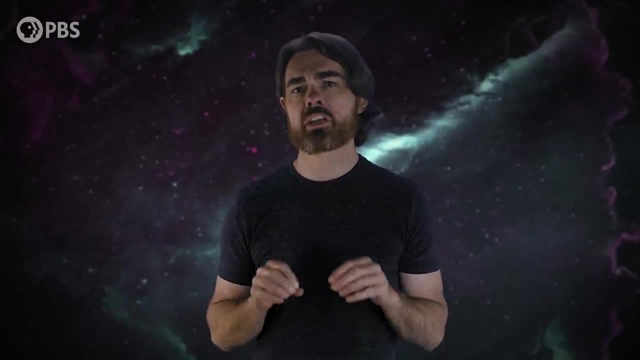 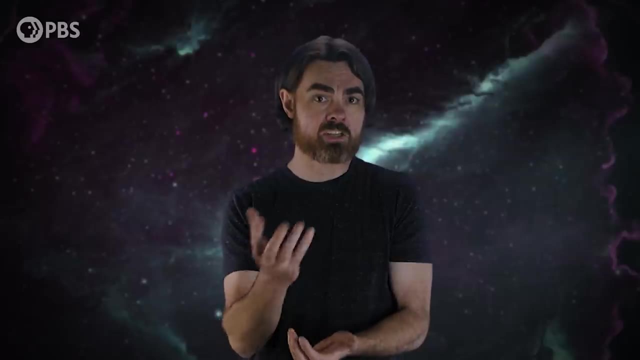 Loop. quantum gravity is a good example, But for that to work, the underlying grid is not a grid of space at all. It's a grid of abstract connections between points. Space emerges only on larger scales. F asks a question which I wish I'd had time to discuss during that episode. 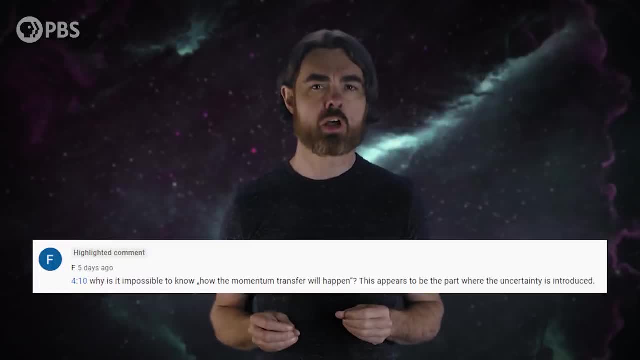 When using the Heisenberg microscope to measure position, I said that the uncertainty in the final momentum of the particle is roughly equal to the momentum of the photon used to measure that position. F points out that surely we should have some idea how that momentum transfer should happen. 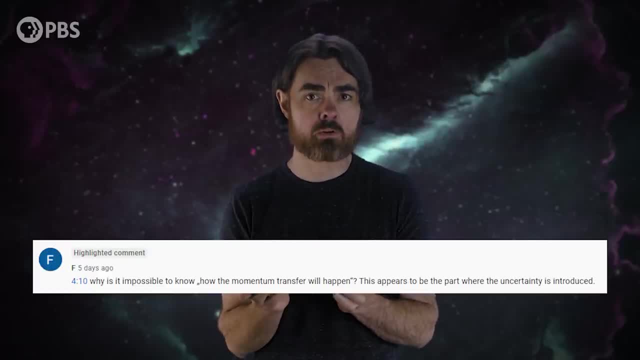 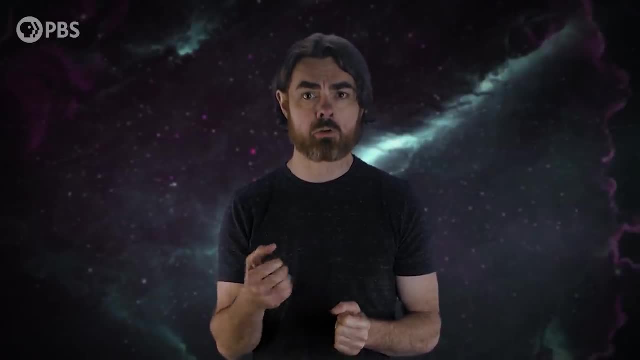 and so should be able to calculate the final momentum of the particle. And if so, then where is the uncertainty? Well, the answer is that there's uncertainty in how the photon hits the particle: Dead on A glancing blow to the left or right?